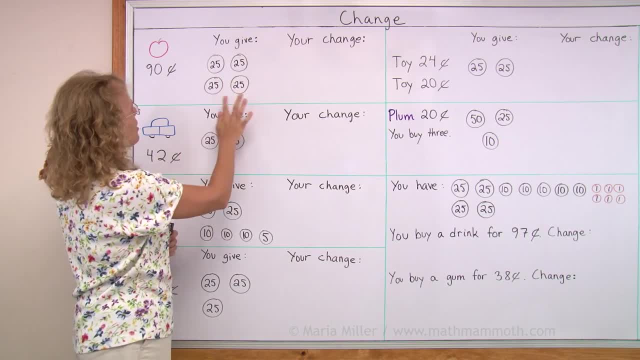 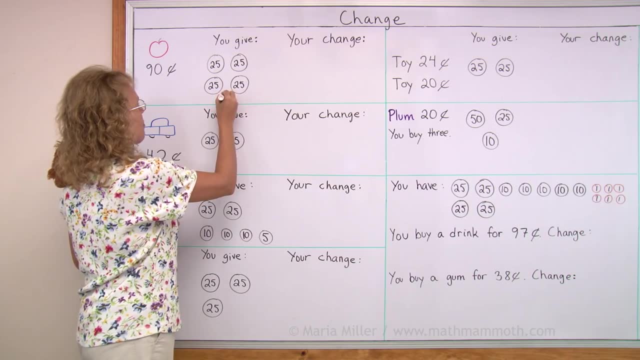 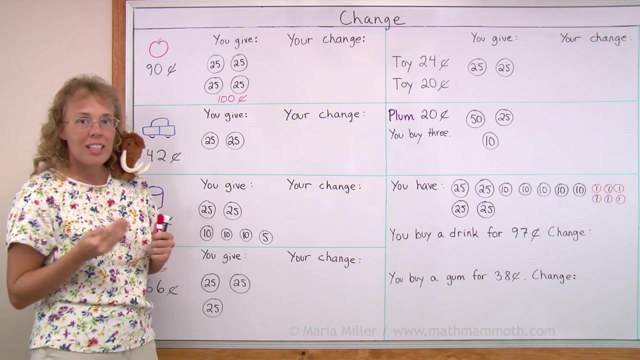 .4 quarters. So how much is this, Do you remember? Four quarters makes hundred cents. Let me write it here. So you're overpaying, You're paying too much, right? And then the clerk will give you back ten cents. That's your change. That is the difference between. 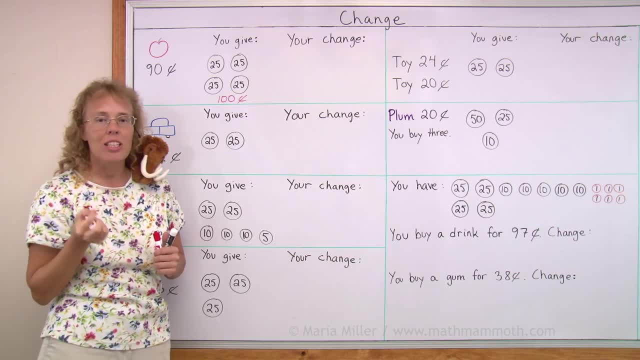 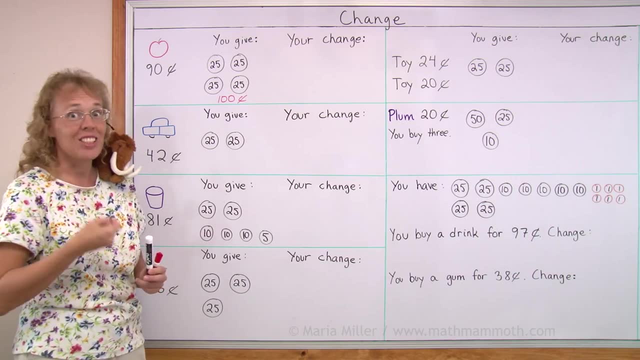 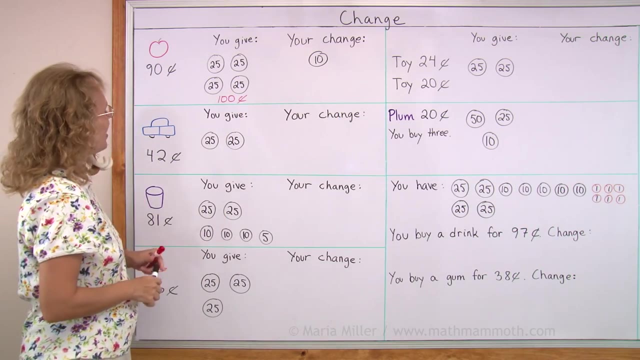 these two 90 cents, hundred cents. It is the amount that you overpay. You pay ten cents, much so. the clerk gives you 10 cents back. that's your change and i'll draw it here as a 10 cent coin, a dime. okay, how about? here? you buy a toy car and it is 42 cents. its price is 42 cents you give. 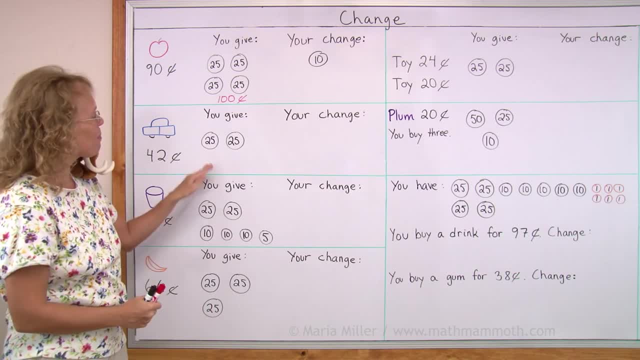 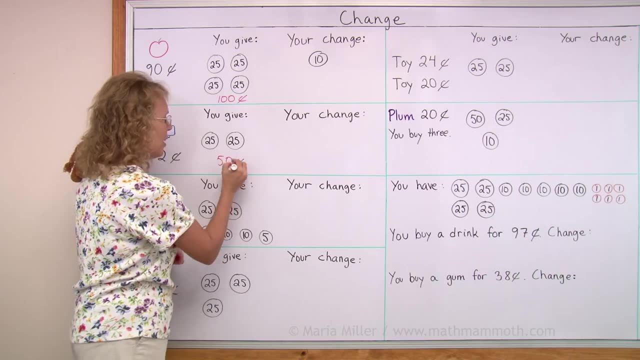 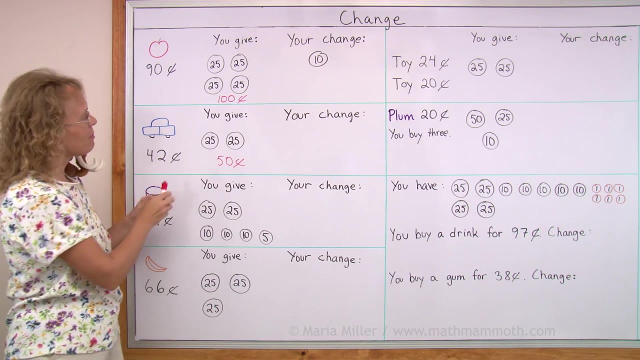 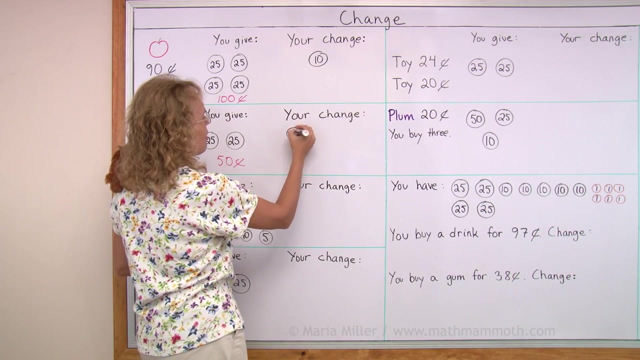 this much because you don't have 42 cents. exactly 25 and 25, that is 50 cents, right? so how much are you overpaying? what's the difference of these two numbers? it is eight cents. so the clerk will give you back eight cents, or of course it has to be five. a nickel and then three pennies- eight cents. 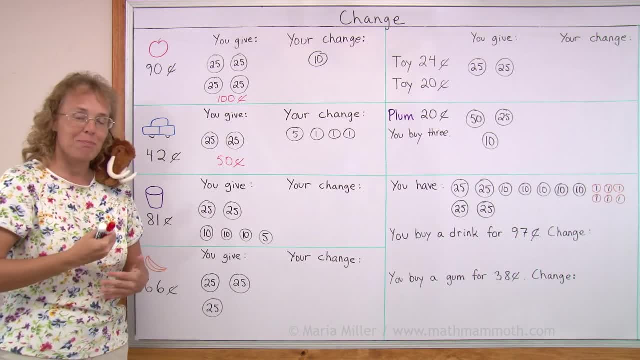 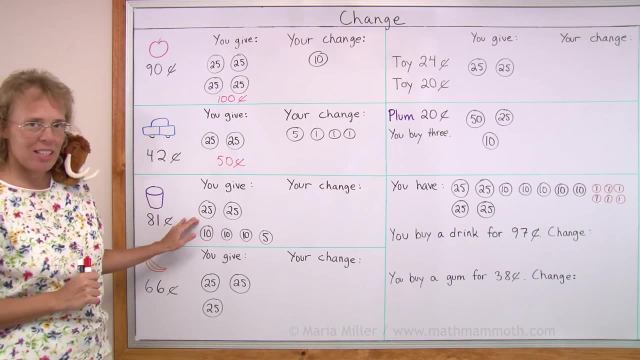 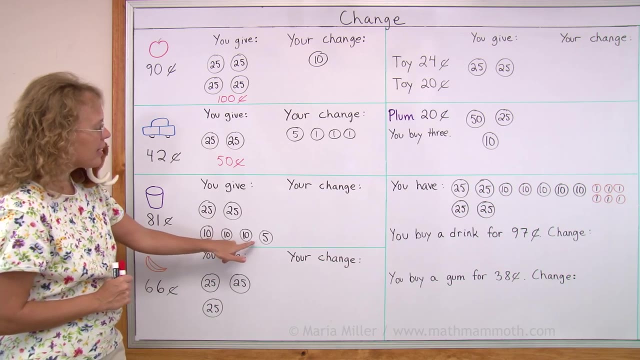 now here's a little bucket for picking blueberries that maybe i want to buy for matthew so he can go pick blueberries. 81 cents, and this is the money i i'm gonna give. these are the coins, so here's 50 cents, 60, 70, 85, 85. okay, let me write it here. 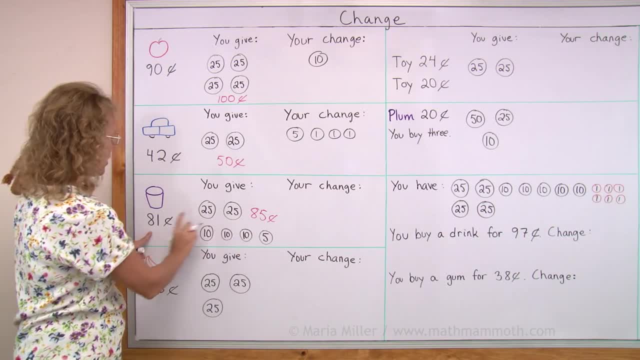 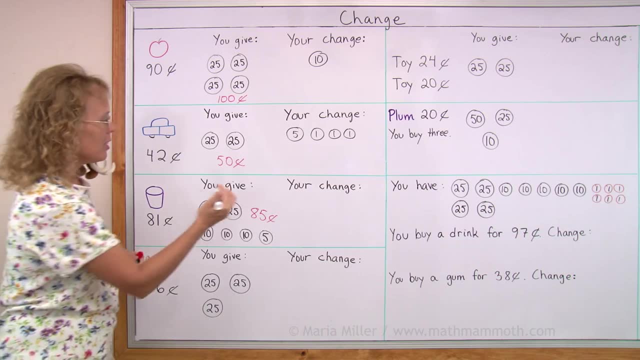 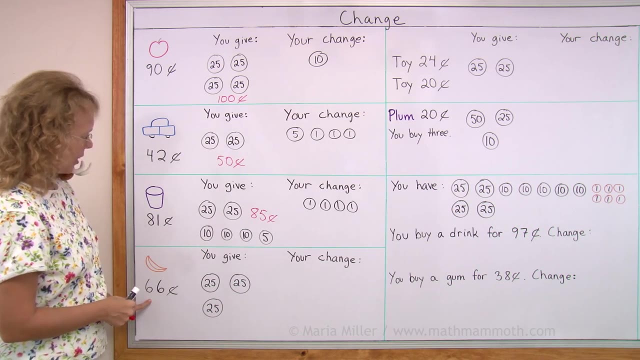 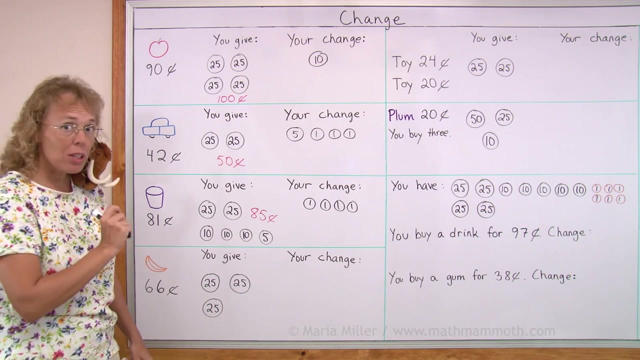 so you can see it. what's the difference here? 81, 85. by how much do i overpay? four cents, right, so the clerk has to give me back four cents, four pennies, and lastly a banana, 66 cents you give. how much is this? three quarters? these two are 50, and then 25, 75 cents. 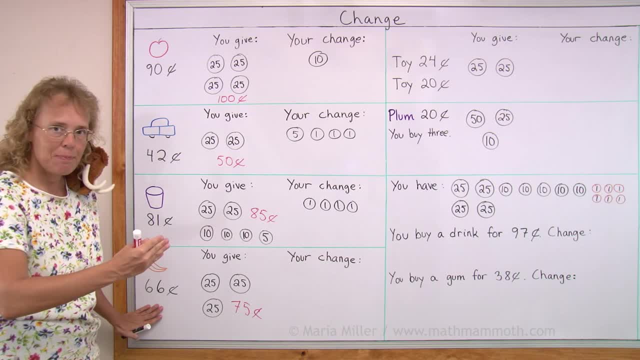 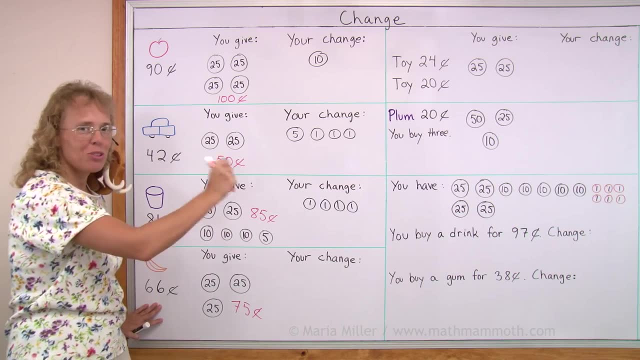 what is the difference now between 75 and 66? if you are at 66 and you want to jump to 75, how many jumps do you need to take? you can think of going from 66 to 70. you can think of going from 66 to 70. you can think of going from 66 to 70. and then to 75. there would be first 4, then 5. the difference is 9 cents. so to make 9 cents you will need a nickel and then pennies for pennies over here. let's say, you buy two toys. one cost 24 cents, the other one cost 20 cents and you give. 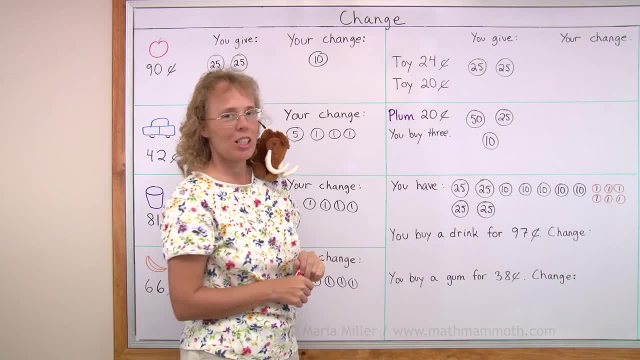 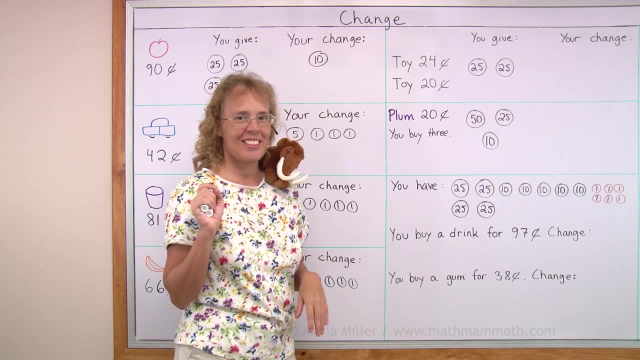 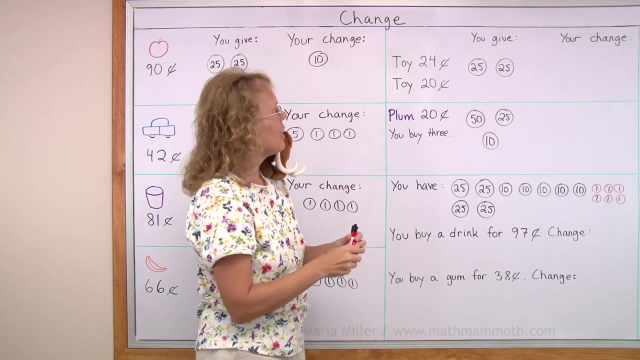 this much money to pay, how much will your change be? we need to first figure out something. what we need to figure out: how much is your total here when you buy those two things- 24 and 20- you add those and you get the total. it is 44 cents. 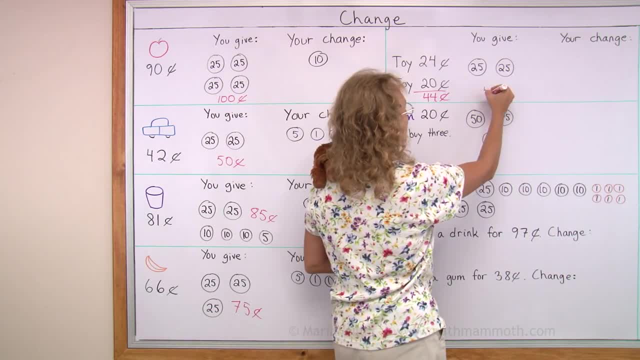 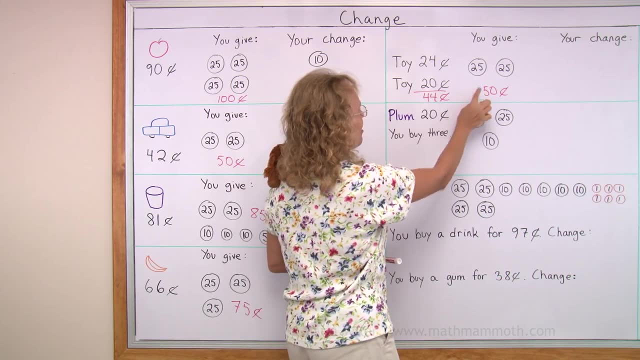 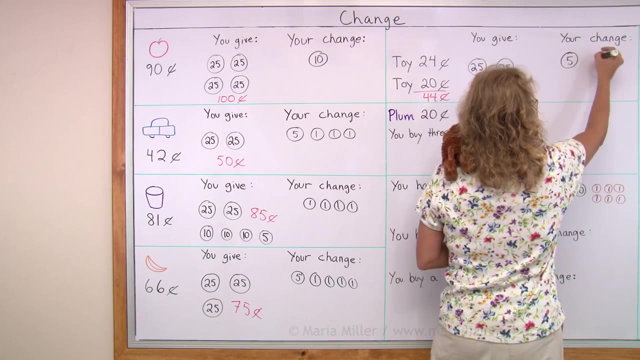 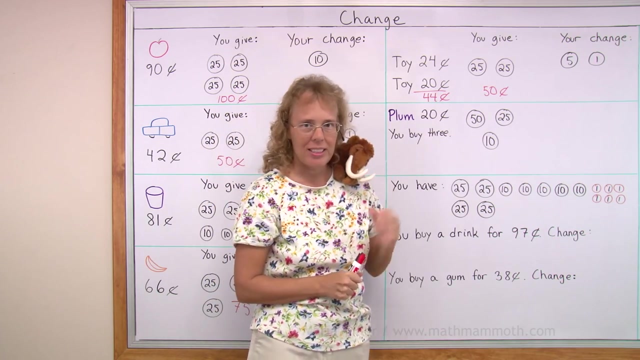 right. and then you give two quarters, which is 50 cents, and now you can figure out the change: 44, 50. how much is there in between, so to speak? 6 cents, yeah, so five. or nickel and a penny, a plum cost 20 cents and Matt is asking: why not blueberries? he 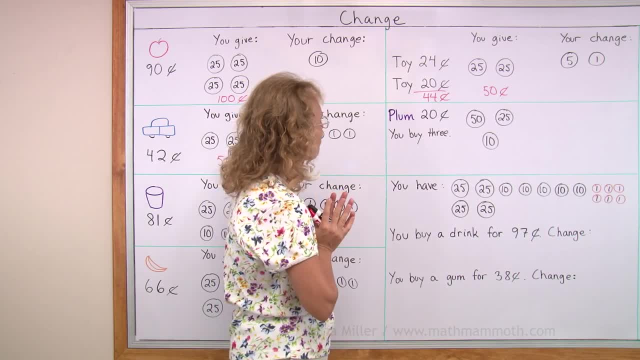 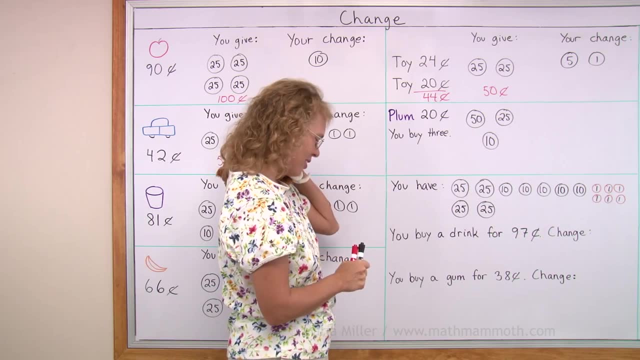 wants to eat blueberries? well, maybe, but how much would one blueberry cost? I don't know. plums are just so much bigger and yummier. I don't know. plums are just so much bigger and yummier. oh, you like them too? okay, that's okay, that's good plum- 20 cents, you buy three. 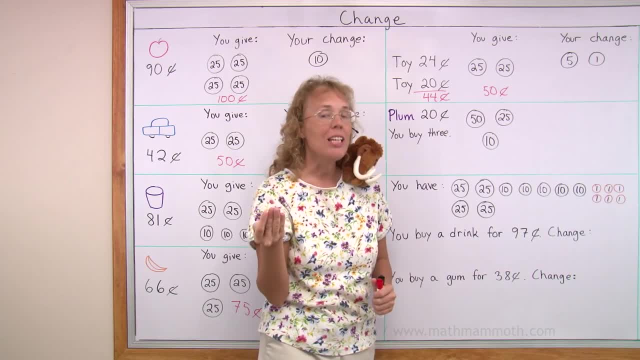 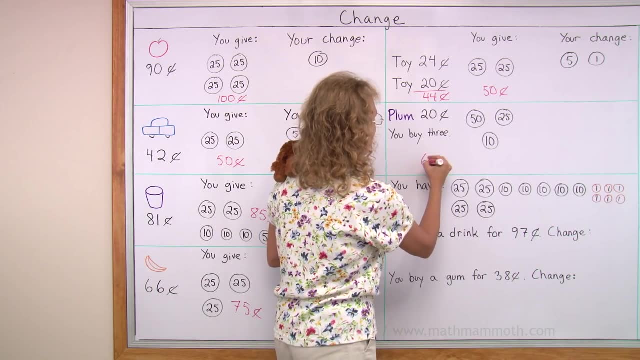 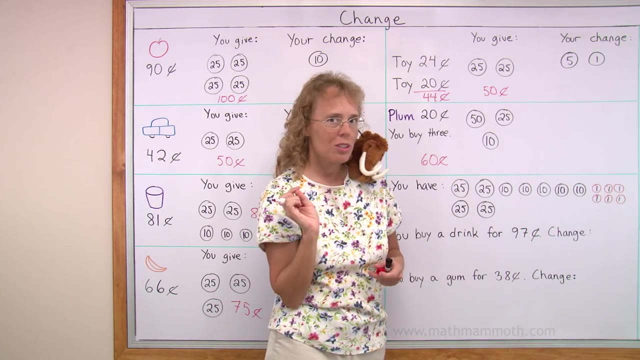 so what is your total cost? three plums: 20 cents each. yep, it's gonna be 20 plus 20 plus 20 is 60 cents. and then how much are you giving here? 50, 10 and 25. so what's your change? 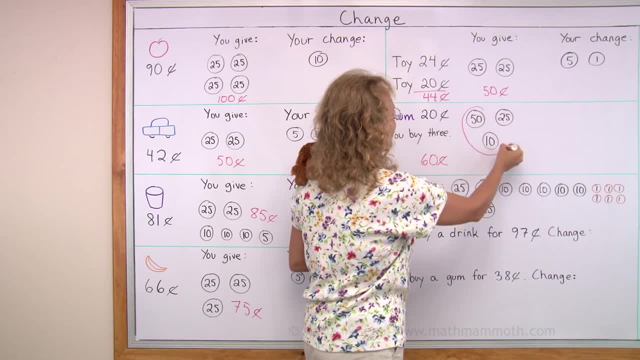 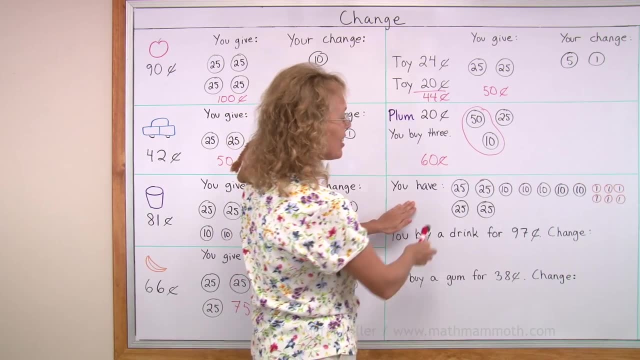 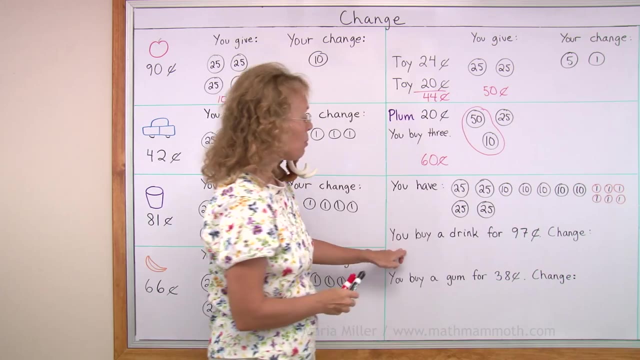 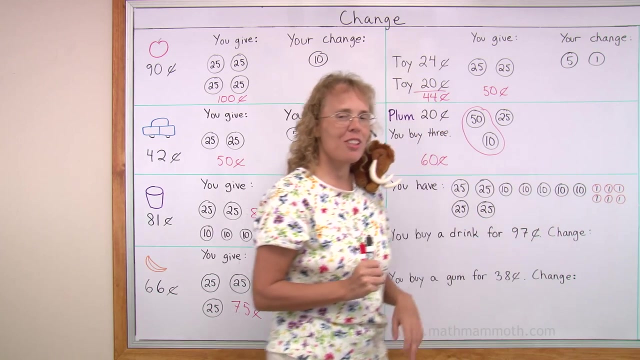 over here. you basically give this and this. you have the exact amount, so you will get no change. okay, here is the coins. here are the coins you have. okay, you go shopping and those are the coins in your purse. let's say you buy a drink for 97 cents. what will be your change? can you figure that one out? 97 cents. 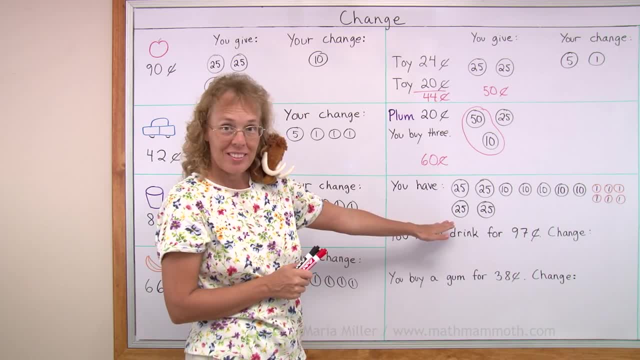 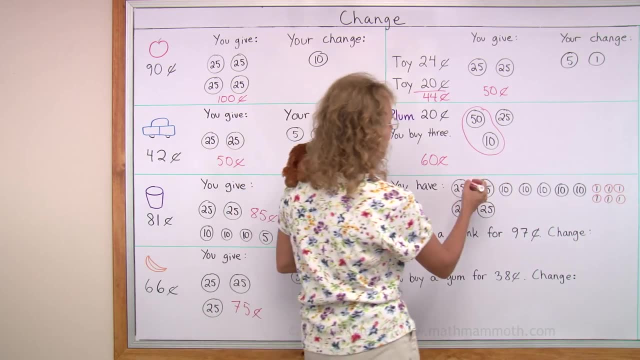 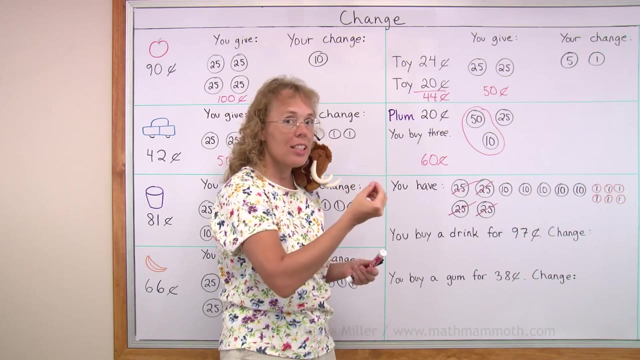 what's your change? Which coins would you give? Okay, this is very close to 100 cents, right? So let's say you give these because these four quarters makes 100 cents, So you give 100 cents. It costs 97, so you change.